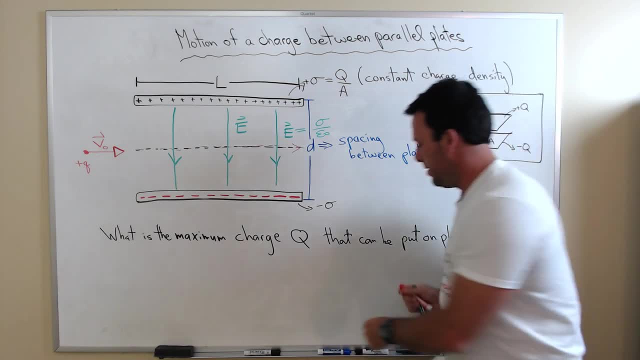 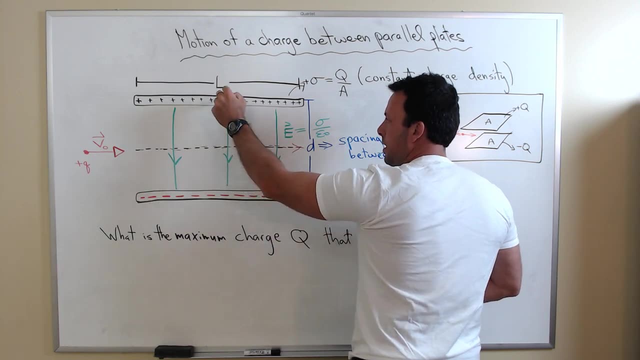 to be a force acting on the charge. The force acting on the charge again, since it's a positive charge. a positive charge in a field that points from the top plate to the bottom plate. as soon as it enters the field region, there's a 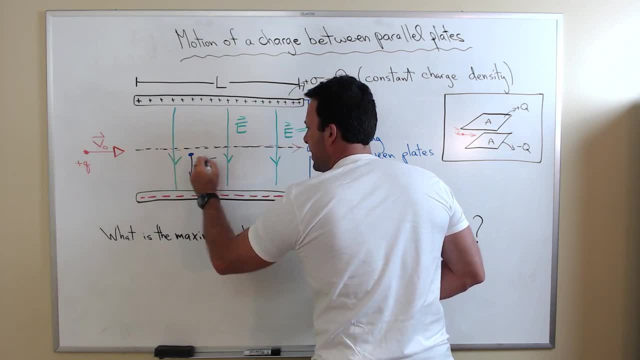 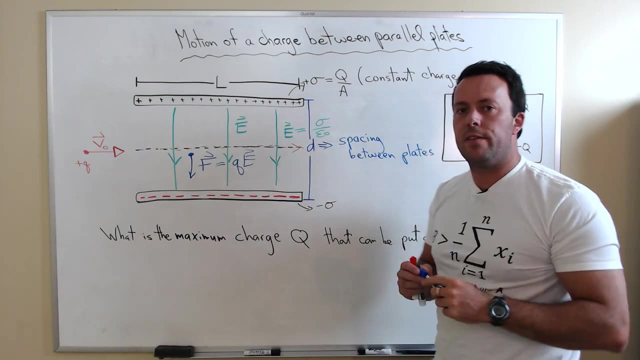 force acting on it. There's an electric force, F, acting on it and the value of the force is simply the magnitude of the charge times the electric field in that region. So this is kind of a special case If the field is very, very big. 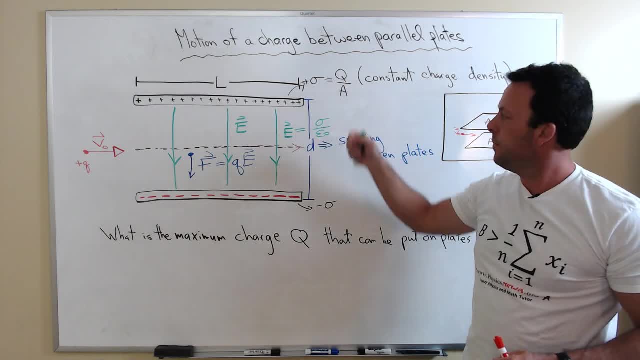 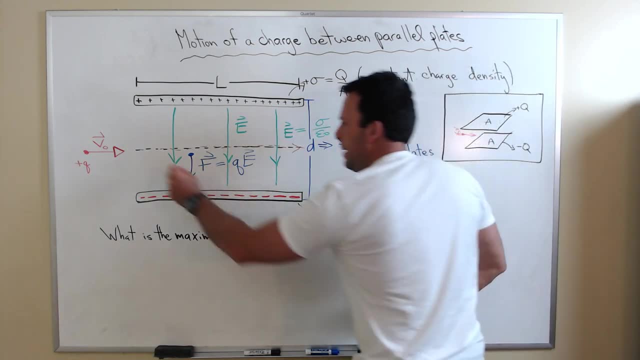 and the field will be very big if you have a lot of charge on it. If I have a very large charge density, the field produced between the plates is going to be very, very big. Well, what's going to happen now is the charge is going to 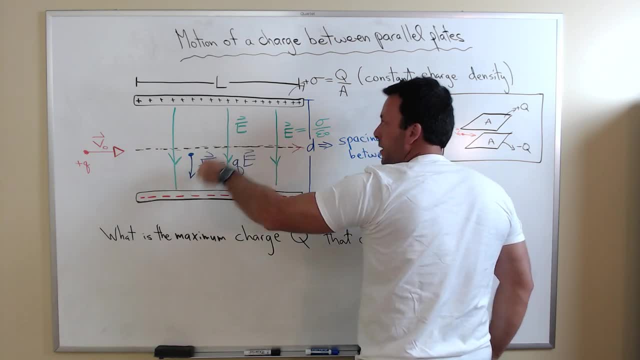 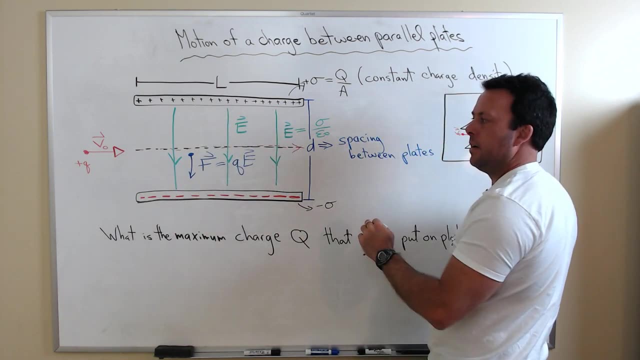 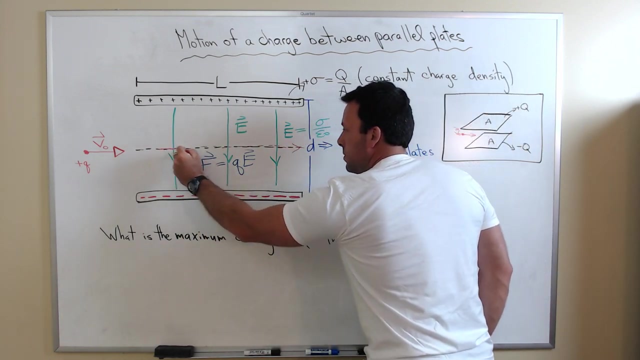 enter this region and there's going to be a large force on it. There's a repulsive force from the positive plate acting on the positive charge and there's an attractive force on the positive charge going through this region. So, if the field is very, very big, this is what it's going to do. It's 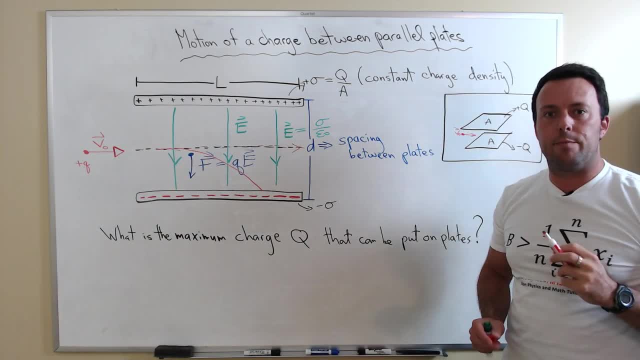 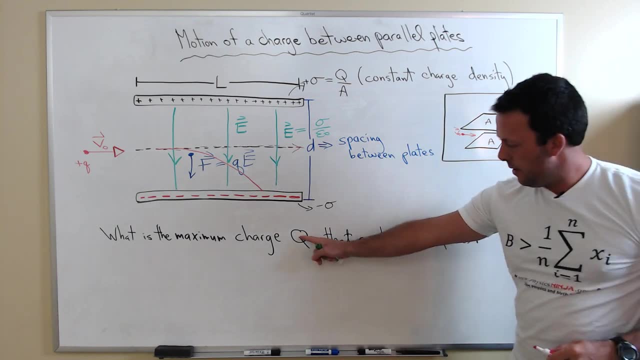 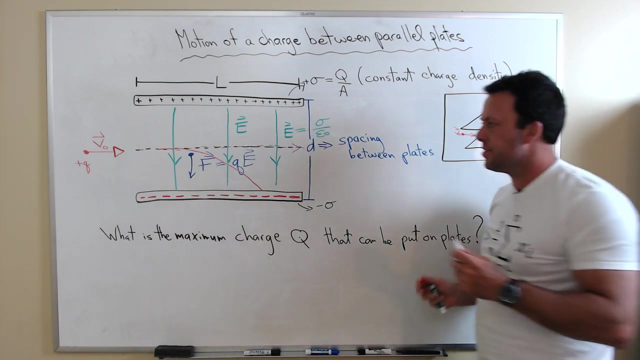 simply going to curve downward and eventually hit that negative plate. Well, we don't want that to happen. okay, The question is: what is the maximum charge, big Q, that I can put on the plates so that I have the maximum deflection of that positive charge? So, if you think, 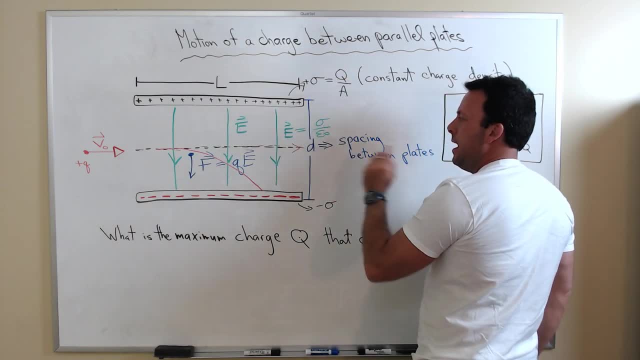 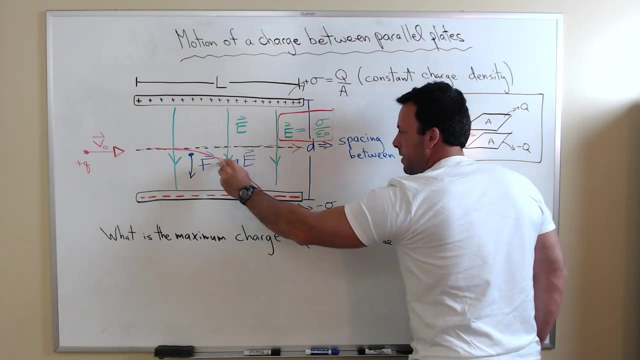 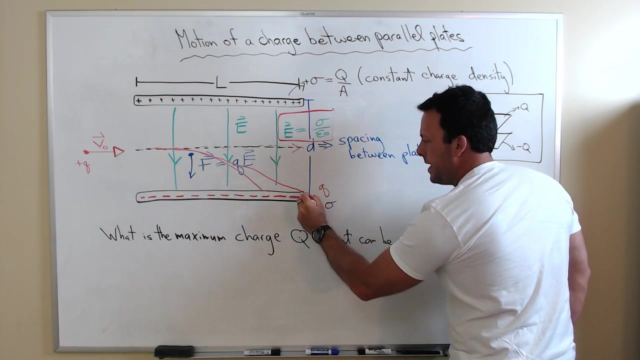 about it. if I put just the right amount of charge on these plates, I'm going to generate just the right electric field such that the charge particle, as soon as it enters the region, starts getting deflected. and if it's just right, I'm going to get this maximum deflection and the little charge Q is going to exit the 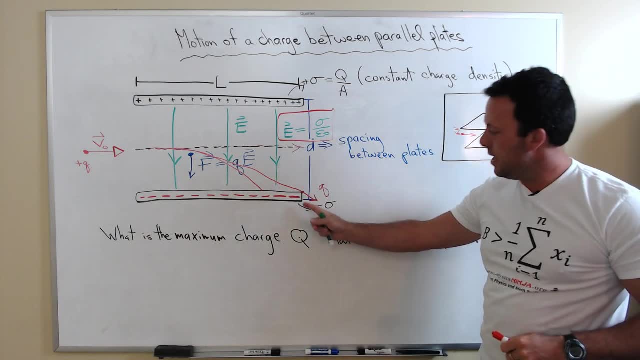 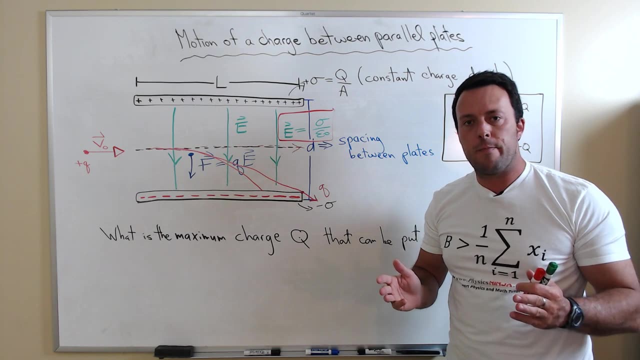 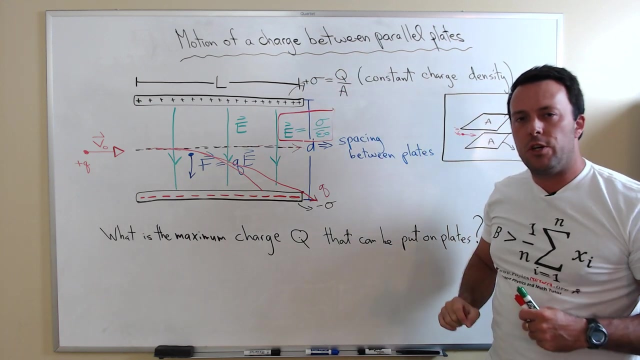 field region at some particular angle. It's not going to hit the plate and it's not going to go straight. it's just going to be the maximum deflection that you can have for that particular charge. So let's go to the whiteboard and see how we can calculate what value of uppercase Q I. 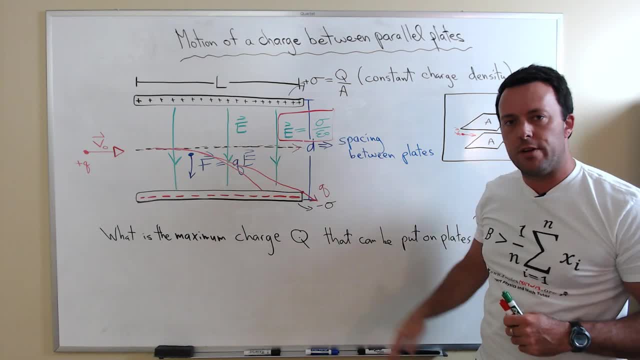 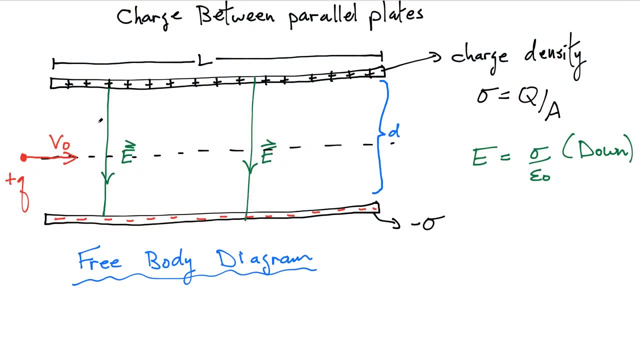 need to put on the plates in order to have this maximum deflection for this small charge moving through that region. Alright, so here's our problem. we have our charge moving into the region where the field is. The first thing you should do is consider a free body diagram. We want to analyze the motion, so let's look. 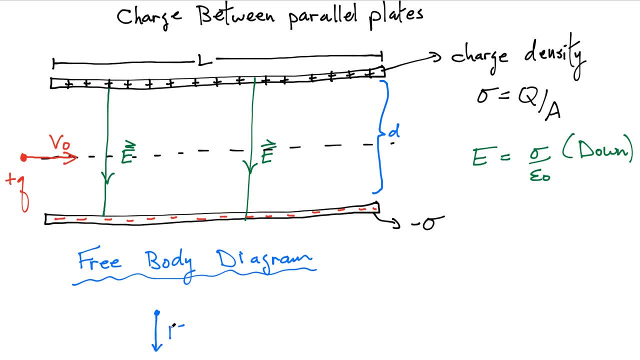 at the forces again, There's only a single force acting on it, that's the electric force. The magnitude of the force is simply Q times the magnitude of the electric field. Since there's only one force, Newton's second law says: you add up all. 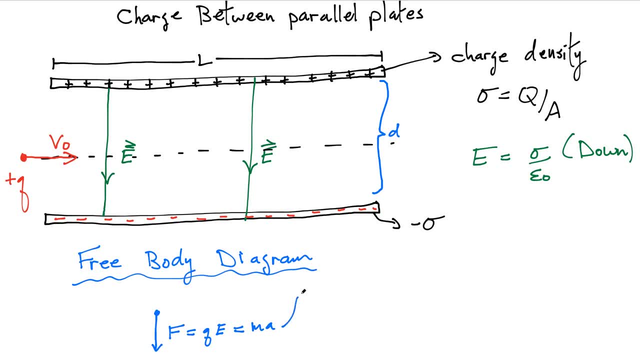 the forces, those should be equal to ma. So the nice thing is, now we have an expression for our acceleration and we simply have QE divided by the mass of the particle. Alright, the nice thing about this: this is a constant acceleration, and that means that means now that we can use all our kinematic equations in order. 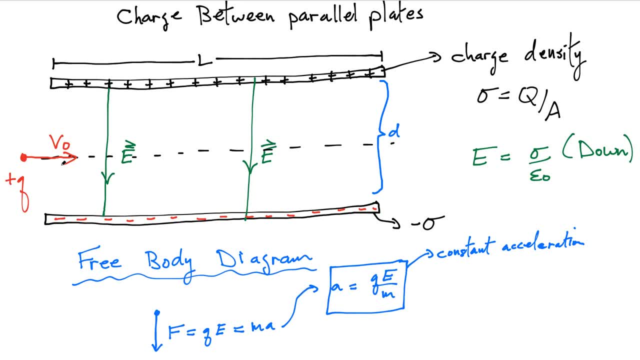 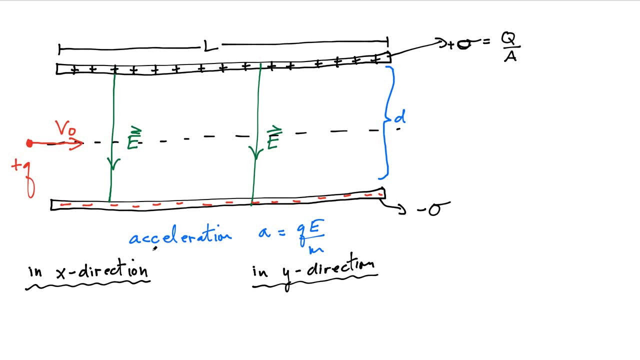 to analyze the motion of this charged particle between the plates. So let's go to the next page and see how we would do that. Okay, so now let's look at the kinematics in the x-direction. Well, in the end, the record in the x-direction- we 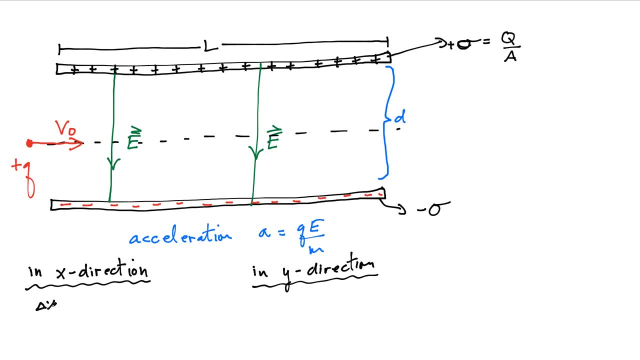 want to look at the displacement in the x-direction. Call that Delta X, and that's simply going to be equal to the initial velocity in the x-direction, which is V naught times the time. The other quantity we want to know during the trajectory is the velocity in the x-direction at any. 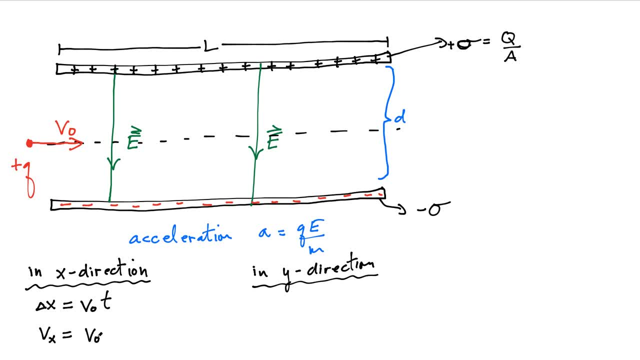 time, and that's simply going to be equal to the initial velocity. There's no acceleration in the x-direction in this problem, because the electric field is constant, the electric force is constant, so that's it. Let's look at now in the y. 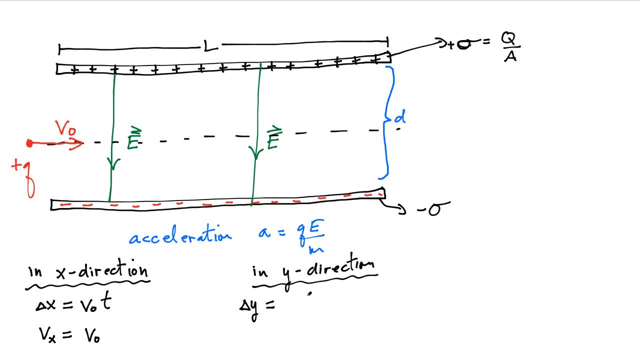 direction. Our displacement y is going to be equal to what? do we have Our initial velocity in the y-direction? There is no initial velocity in the y-direction. Okay, so that term vanishes. So typically you'd have a term like this: and if we define a coordinate system where positive x is this way, and let's 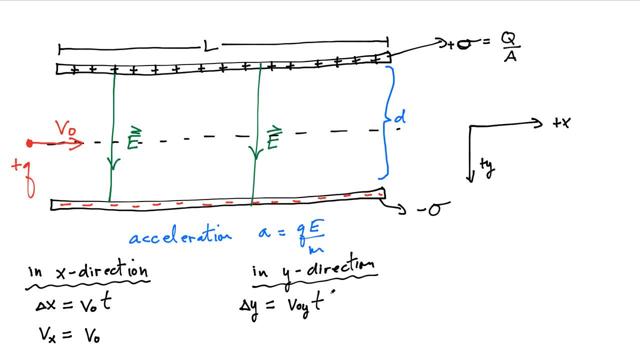 make positive y in this direction, so our acceleration will be positive. We have another contribution here, which is one half a t squared. However, this term, as I mentioned, is going to be equal to zero because there is no initial velocity. Initially, I'm just going. 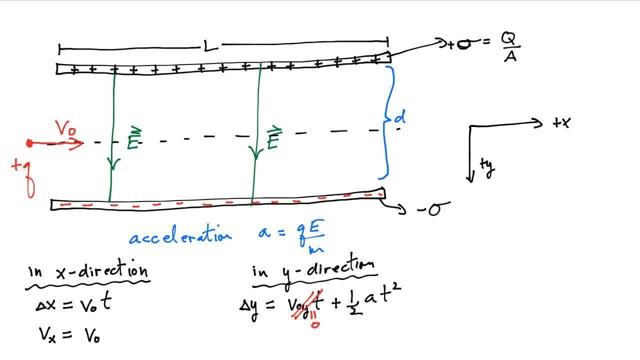 along the x-axis. The other thing I want to know is what is the velocity at any motion, at any point in time in the y-direction? Again, it's the initial velocity in the y-direction, which is zero, and we can't forget our acceleration. 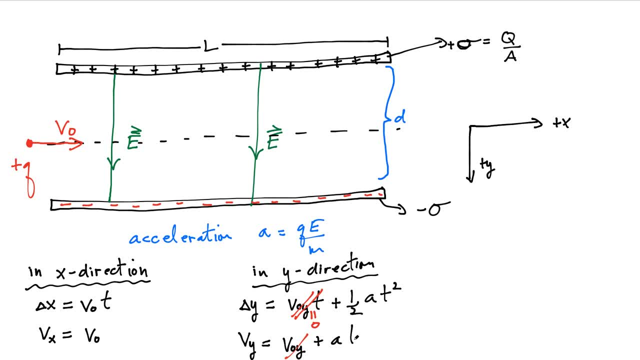 term plus acceleration times time. Okay, there you have it, folks. So we have kinematic equations that tell us the x-displacement, the y-displacement and the velocity components at any instant in time. So now we can go back and analyze the problem and find what we're. 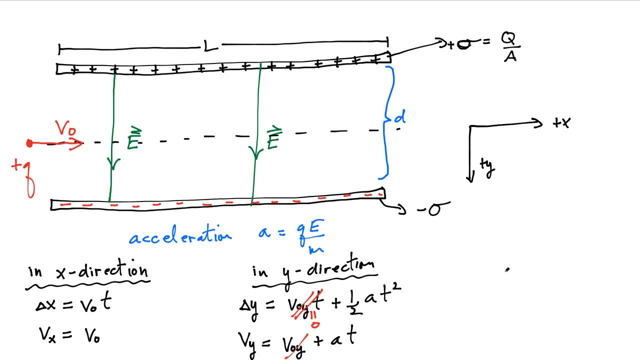 looking for. So this problem is exactly identical to throwing an object horizontally from a cliff and you want to see how far it goes. We want the range in this particular problem, so the distance it travels to be the distance of the plates, or the length of the plates, which is L, and we're going to want to set. 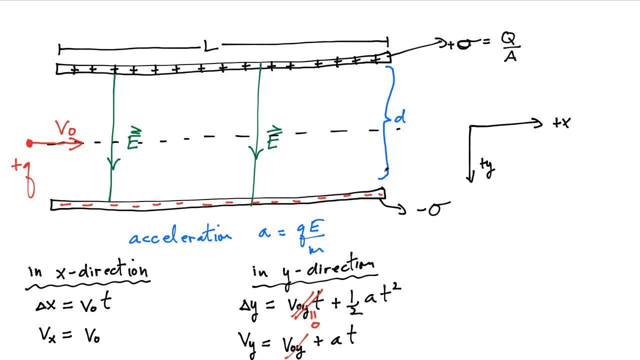 our y-displacement to be the maximum value. When the y-displacement is equal to d over two, we're going to get the maximum deflection of this charged particle when it goes through the plates. So let's go to the next page and set that problem up. Okay, so we want. 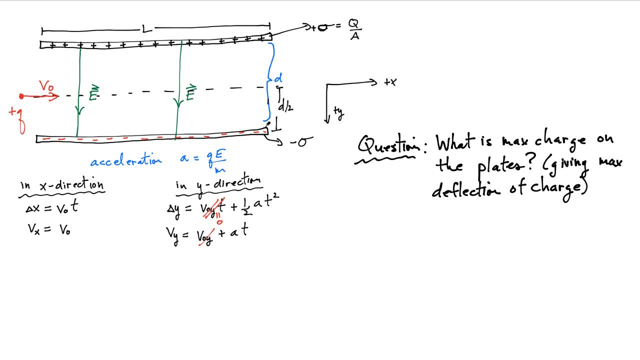 our maximum deflection. We want to calculate what the maximum deflection is going to be. Well, all we really need to do is we really need to set the y-displacement equal to half the distance between the plates, because I'm starting already at the midpoint, So I really want my y-displacement to be d over two, and 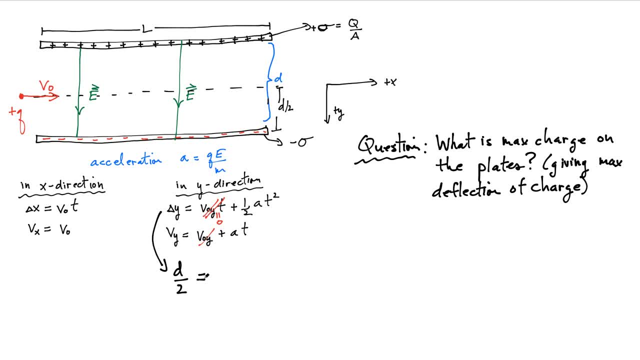 positive d over two, because the displacement is down, That there is going to be equal to one half. What is my acceleration? The acceleration I can write it in terms of the field qe over m over multiply times t squared. Therefore, I still have the time on this equation. So 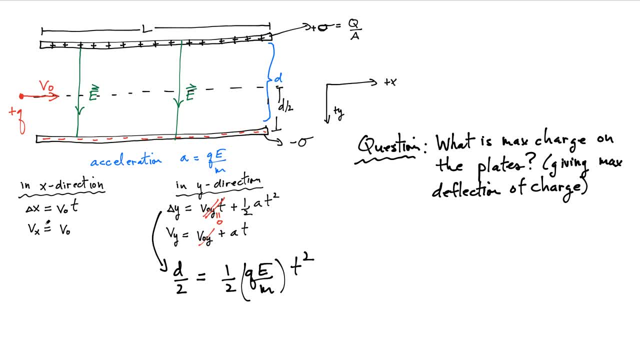 I need to find a way to eliminate the time, and in order to do that, I can use my x-displacement, because, really, what I want to do is I want this maximum displacement to be when the particle is just exiting the plates, and that's going to be when my displacement in the x-direction. 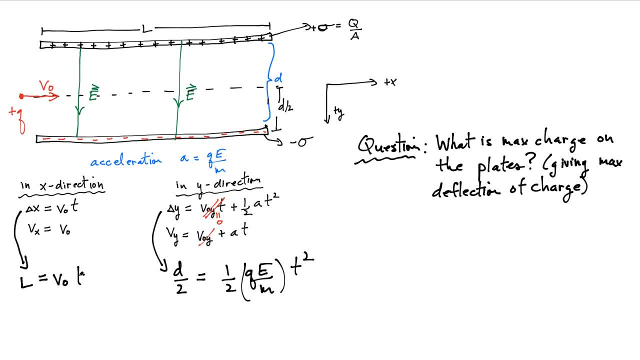 is equal to L. Okay, Okay, Okay, Okay. When do I have that? I'm going to have. the displacement is going to be equal to the length of the plates when the time is simply L divided by my initial velocity. So if you go ahead and substitute that into our equation over here for the Y displacement, 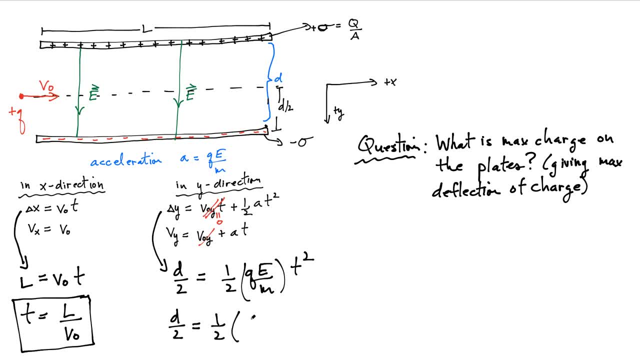 we get D over 2 equals to 1 half QEM and we're going to have L over V, naught squared. So this here is the maximum displacement and this here is really going to be the maximum electric field that's going to give me that displacement. 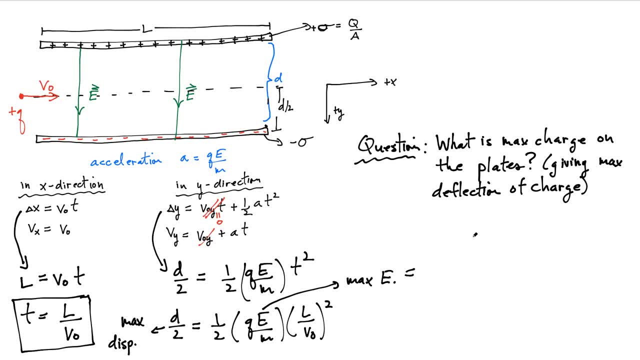 Okay, So I can actually just isolate for that. and what do I get? Well, the 1 half terms cancel out. I'll just do a little bit of algebra and simplify So the maximum electric field that I'm going to get. 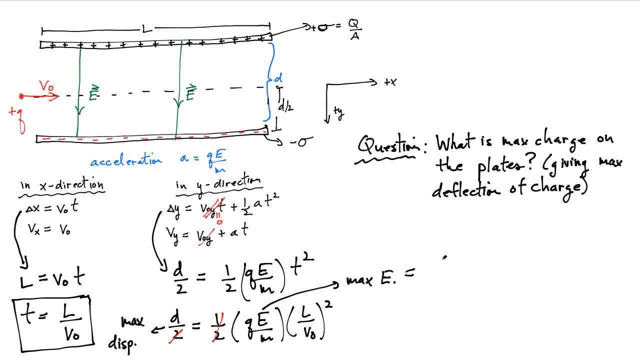 or that will produce the displacement. the maximum displacement is going to be MD. make sure I do things correctly here. divide through by the charge and then I have to eliminate this term, the L over V naught term. If I bring that over to the other side, it becomes V naught over L and it's still squared. 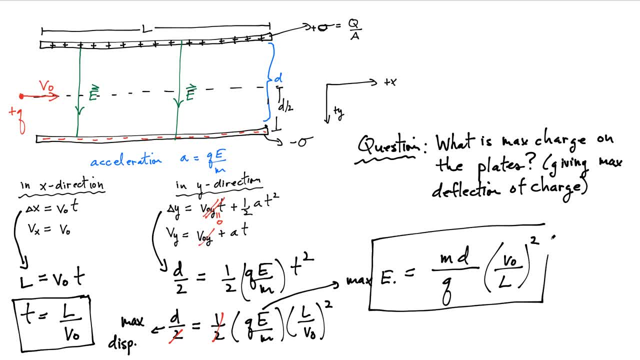 So here's the maximum value of the electric field. Now the question was posed a little bit differently. I asked: what's the maximum charge on the plate? Well, that's very easy, Because we're looking at parallel plates and the field produced by parallel plates. 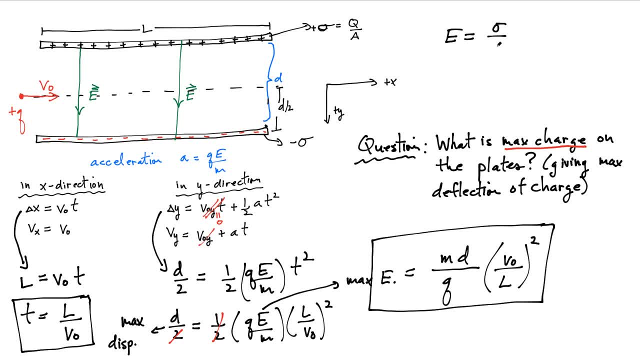 at least in the region between the plates, is sigma divided by epsilon zero, Okay, And the sigma is simply the surface charge density. It's the amount of charge you have per unit area of plate, and we still have the epsilon zero constant. 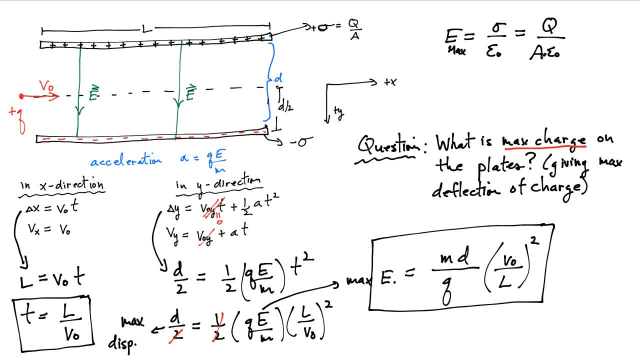 So the maximum electric field is going to be for any given geometry, whenever I maximize the charge density or maximize the charge on the plates. So our last step, putting everything together. now let me make a bit more room here. Okay, So we're going to have Q max.